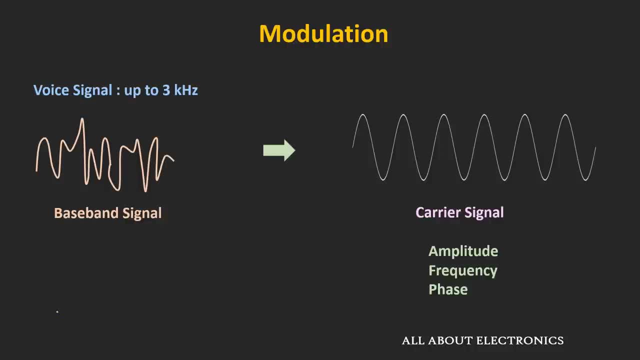 So the modulation is the process where one of the properties of the carrier signal, like the amplitude, phase or frequency, is changed according to the baseband signal. baseband signal And based on the which properties changed, there are different types of modulation. But before that, first of all, let us see why this. 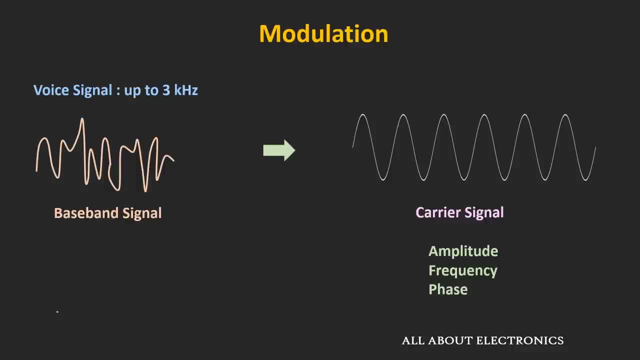 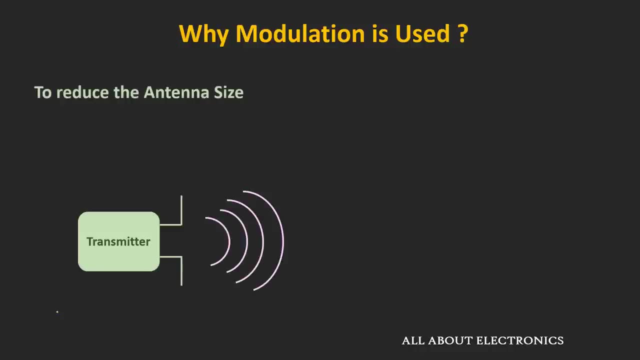 modulation is required. So the first reason to use this modulation is to reduce the antenna size. So when the signal is transmitted wirelessly, then the size of the antenna is very important parameter. So this size of the antenna is proportional to the wavelength of the transmitted signal. And 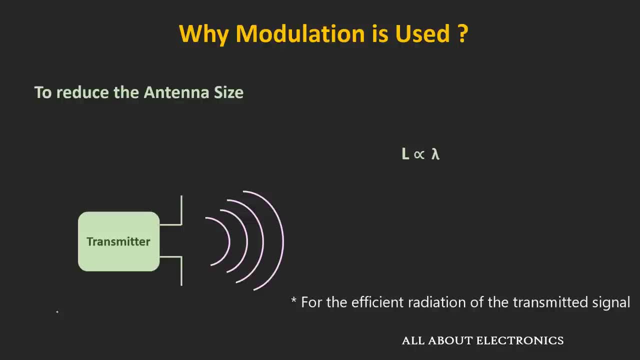 depending on the type of the antenna, it is the fraction of the transmitted wavelength. So let's say the size of the antenna is equal to lambda by 4.. Now the relationship between the frequency and the wavelength can be given by the following expression. So, for example, if the transmitted signal has a frequency, 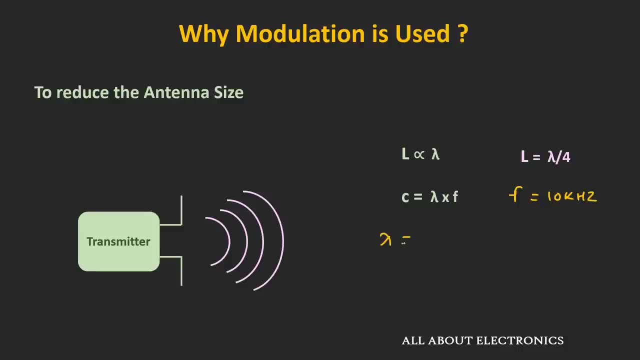 of 10 kilohertz, then its wavelength will be equal to C divided by F. that is equal to 3 into 10, to the power 8 times. So if we calculate the wavelength then it will come out as 30000 m. 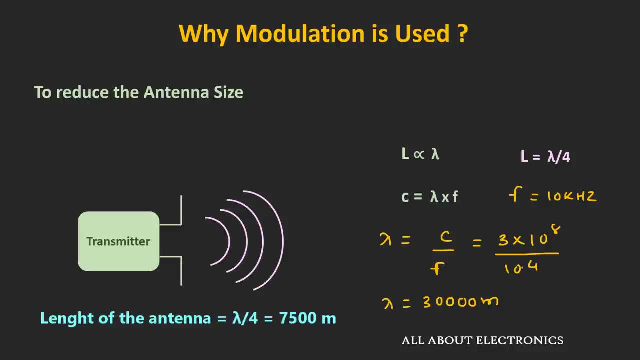 And if the size of the antenna is a quarter of the wavelength, then the length of the antenna will come around as 7500 m, And this size is actually impractical, right. On the other hand, if the signal is transmitted at, let's say, 10 MHz, then the length of the 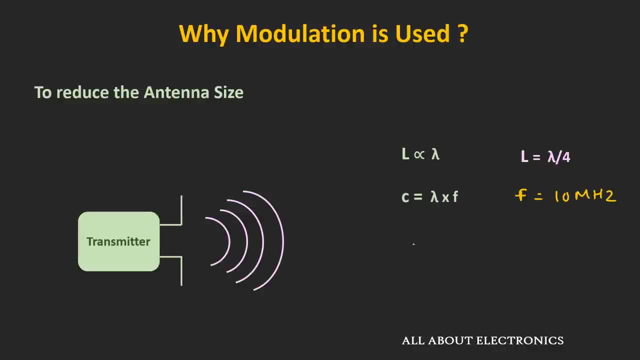 antenna will reduce by the factor of 1000.. That means in that case, the length of the antenna will be equal to 7.5 m, And in fact this size of the antenna is manageable, right. So that is one of the reasons for the modulation. 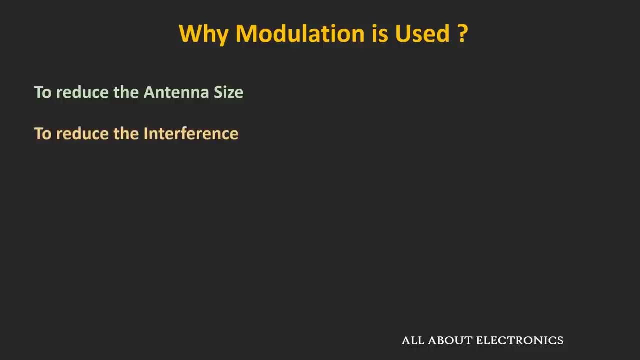 Then the second reason is to reduce the interference. So just imagine in a single room if 3 persons are talking to the same person, then that person won't get anything right. Similarly, let's say if 5 different voice signals which are around in the same frequency 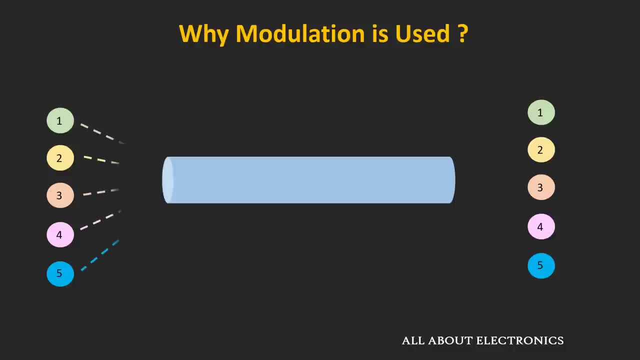 range are transmitted without modulation through a single channel, then there will be an interference between them and at the receiver we won't get the transmitted signal. But instead of that, if each signal is modulated at the different carrier frequency and all carrier frequencies are relatively far away from each other, then there won't be any interference. 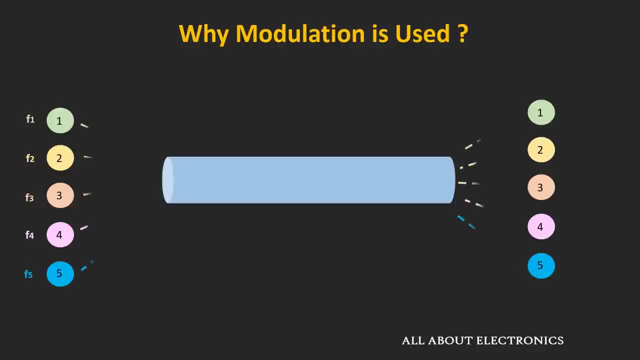 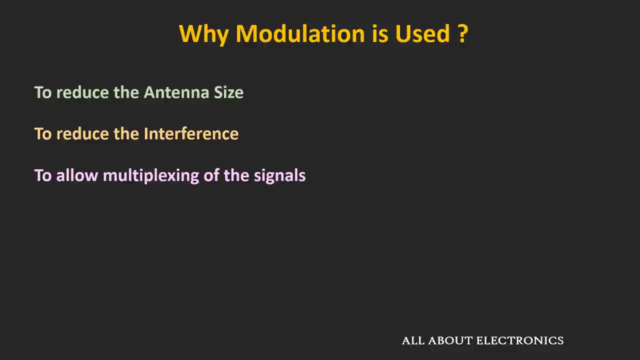 All the signals can be demodulated at the receiver and the message signals of each transmitter can be retrieved. So, using the modulation, the interference can be reduced And at the same time the multiplexing of the different signals is also possible. 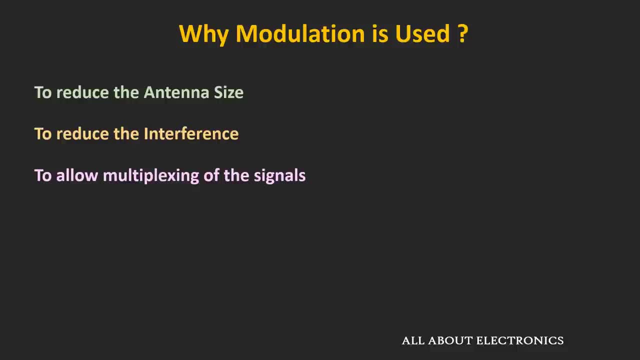 And the example which I showed you earlier is the example of the frequency division multiplexing, where the different message signals are modulated at the different carrier frequencies and because of that they can be transmitted simultaneously. So these are some of the important aspects why the modulation is used in the communication. 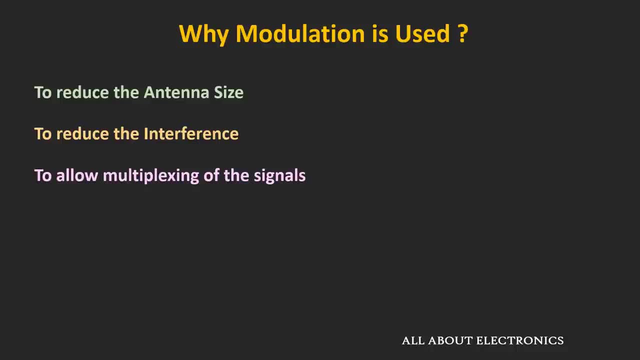 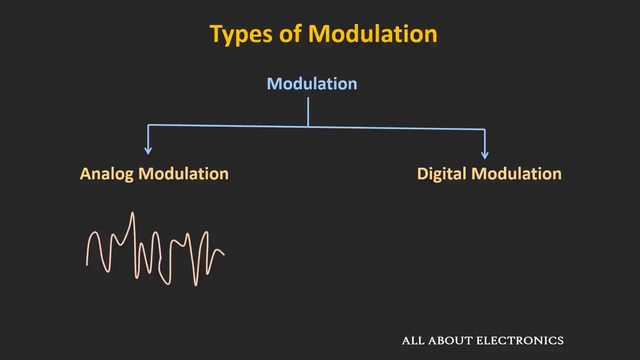 So now let's see the different types of modulation. So broadly there are two types of modulation: The analog modulation and the digital modulation. So if the message signal is analog, then it is known as the analog modulation, And similarly, if the message signal is in digital form or in digital form, then it 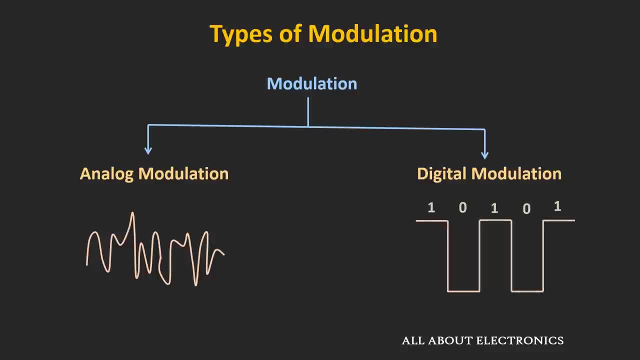 is known as the digital modulation. So first of all let's talk about the analog modulation. So, based on the type of the carrier signal, this analog modulation can be further classified into two categories, that is, continuous wave modulation and the pulse modulation. 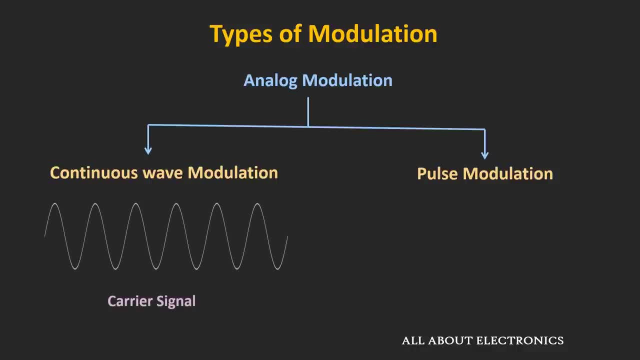 So if the carrier signal is a continuous wave signal, like a sine wave signal, then it is known as the continuous wave modulation. But to supply friction one way or another, one can only thesis the different waveforms. Let's think about it like this: 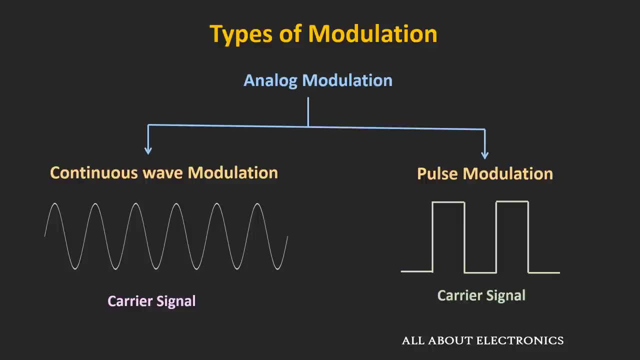 If the carrier signal is a pulse signal, then it is known as the pulse modulation And first of all let's see the different types of continuous wave modulation. So mainly there are 3 types of modulation, That is, amplitude modulation, the frequency modulation and the phase modulation. 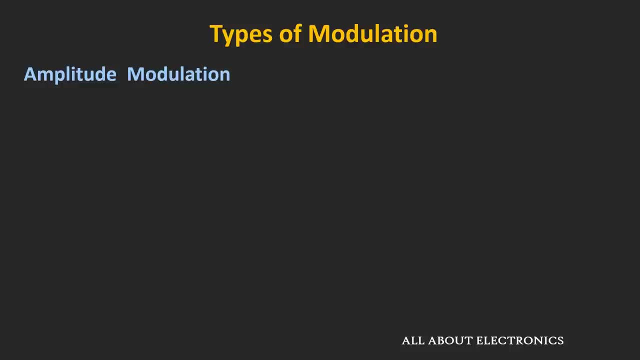 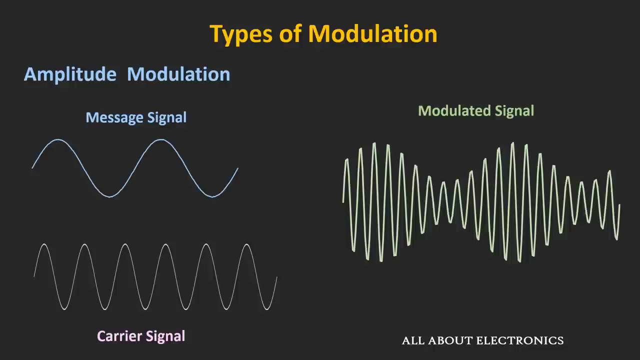 So in case of the amplitude modulation, the amplitude of the carrier wave changes according to the message signal. So if this is the message signal and the high frequency signal is the carrier signal, then the amplitude modulated wave would look like this. So, as you can see over here, the shape of the carrier wave changes according to the 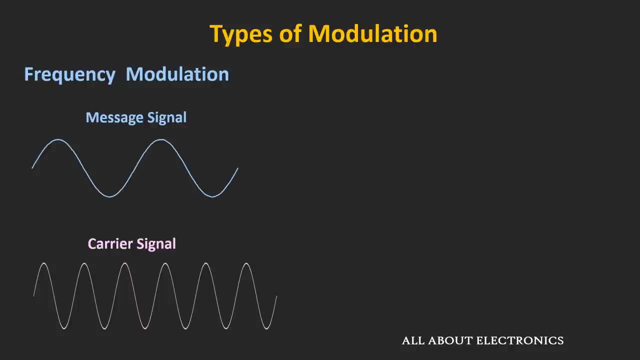 message signal. Similarly, in case of the frequency modulation, the frequency of the carrier wave changes according to the message signal. So with the increase in the amplitude of the message signal, the frequency of the modulated signal will also change. Similarly, with the reduction in the amplitude, the frequency of the modulated signal will. 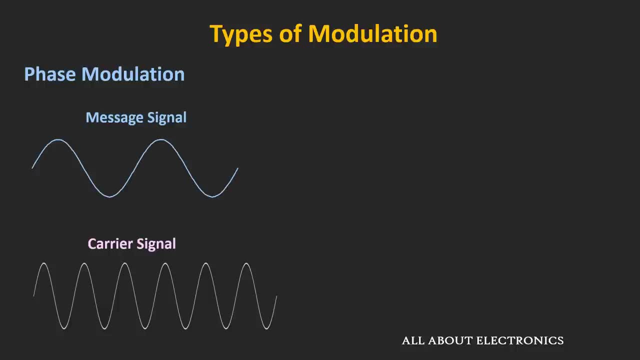 also reduce. And similarly, in case of the phase modulation, the phase of the modulated signal changes according to the message signal. So in the upcoming videos we will talk about all these different modulation techniques in detail. Alright, so now let's see the different types of pulse modulation techniques. 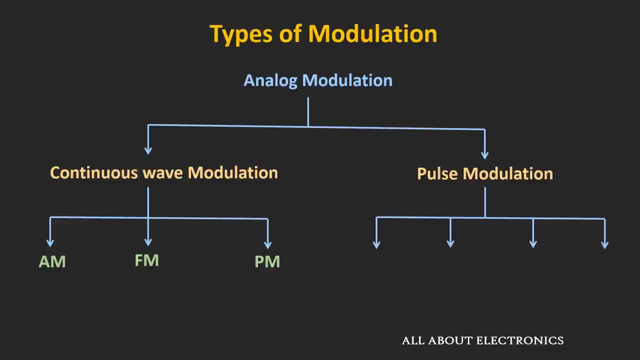 So mainly there are 4 different types of pulse modulation, That is, pulse amplitude modulation, the pulse width modulation, the pulse position modulation and the pulse code modulation. So let's briefly see all these techniques one by one. So in all these modulation techniques the message signal is analog in nature, while the 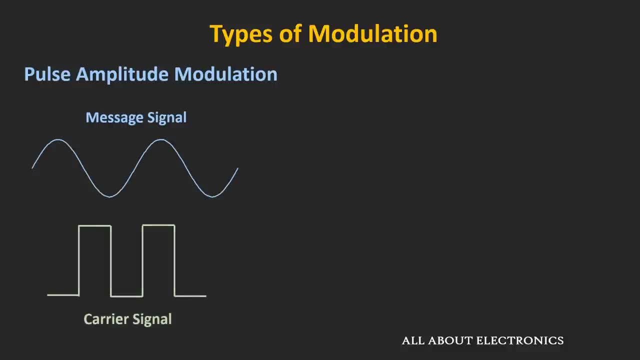 carrier signal is a pulse strain of the finite frequency. So in case of the pulse amplitude modulation, the width or the duration of the pulse will remain same, But the height or the amplitude of the pulse signal will change according to the message signal. Similarly, in case of the pulse width modulation, the height or the amplitude of the pulse will 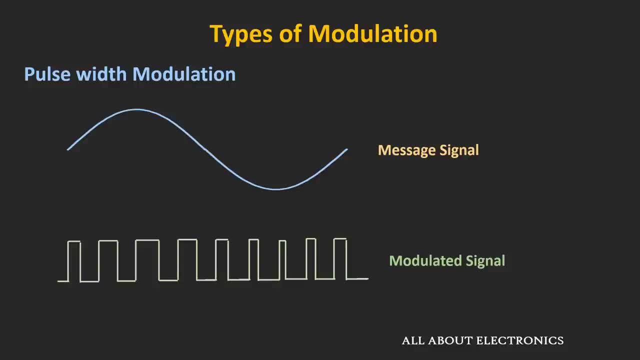 remain same, but the width of the pulse will change according to the message signal. So here the message signal amplitude is sampled at the rising edge of each pulse and the width of the modulated signal is proportional to the sampled amplitude. And in fact, on the pulse width modulation I have already made the separate video earlier. 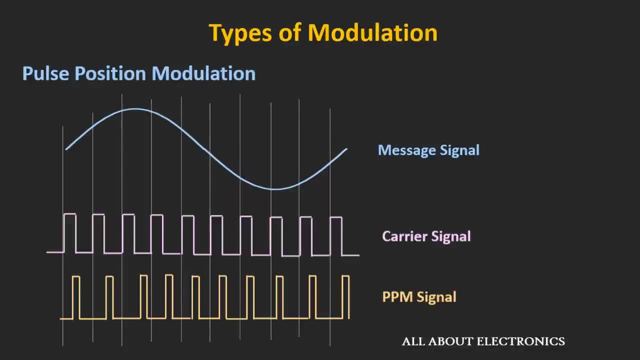 So for more information you can check that video. Similarly, in case of the pulse position modulation, the width and the amplitude of the pulse will remain fixed, But the position of the modulated signal will change according to the input signal. So at each rising edge the message signal is sampled and based on the amplitude of this. 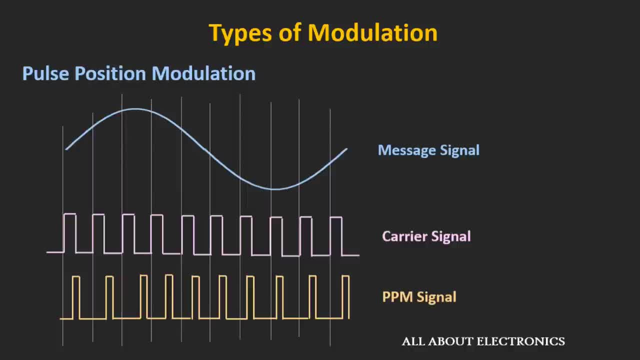 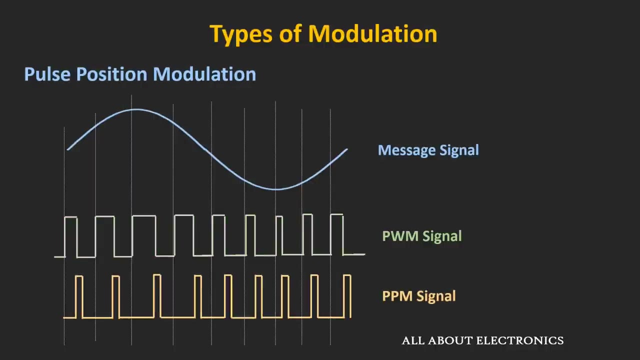 input signal, the position of the modulated signal will change. That means as the amplitude of the input signal increases, then this modulated pulse will further go away from the reference position And in fact it can be generated with the help of the PWM signal. 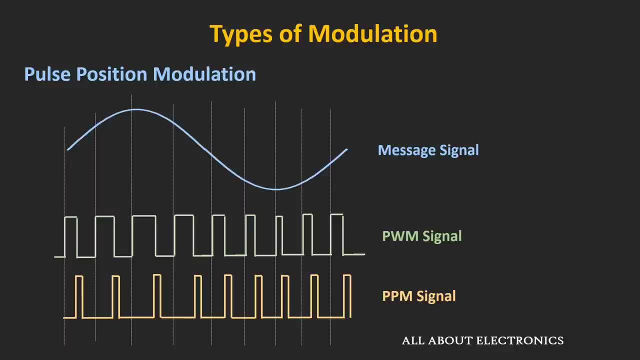 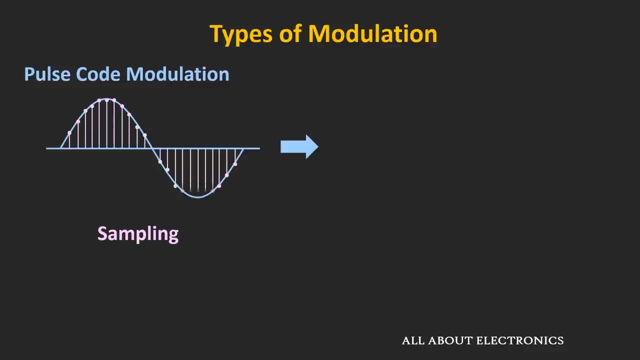 That means, by generating the pulse at every falling edge of the PWM signal, this PPM signal can be generated. Alright. so now let's move to the next modulation scheme. So in the Pulse Code Modulation The message signal is sampled at the finite interval. 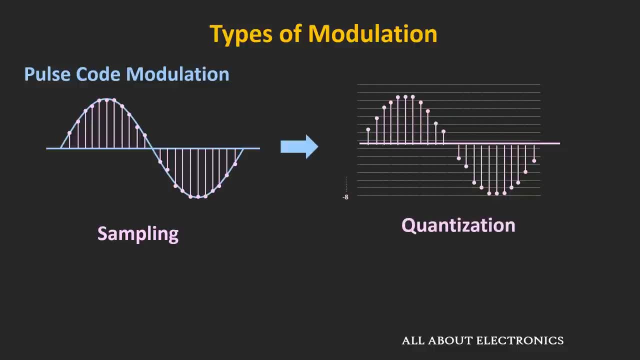 And the sampled value is quantized using the quantization process And then using the analog to digital converter, the message signal is encoded. For example, if the sampled value is encoded in the 5 bits, then for every sampled value we will get a pulse code of 5 bits. 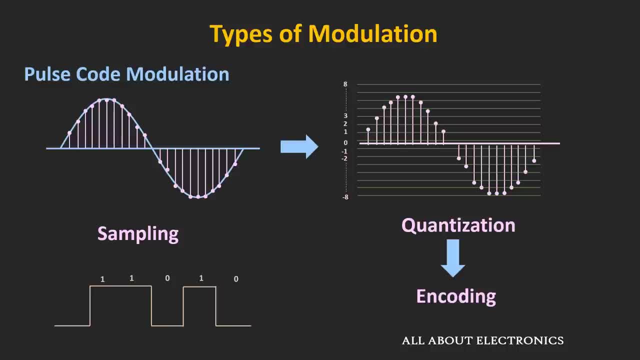 So this is the very brief overview of the Pulse Code Modulation, But in the future videos we will discuss the Pulse Code Modulation. We will see in detail about this. Pulse Code Modulation: Alright, so far we have seen the different types of analog modulation techniques. 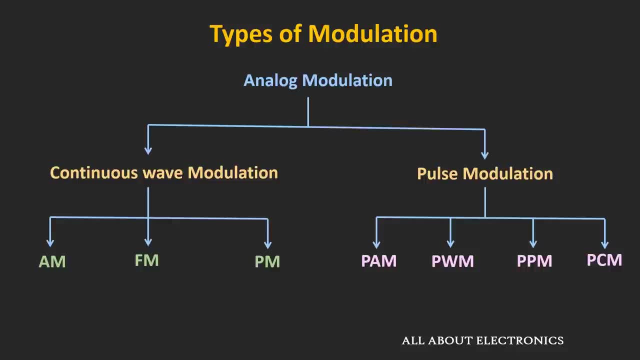 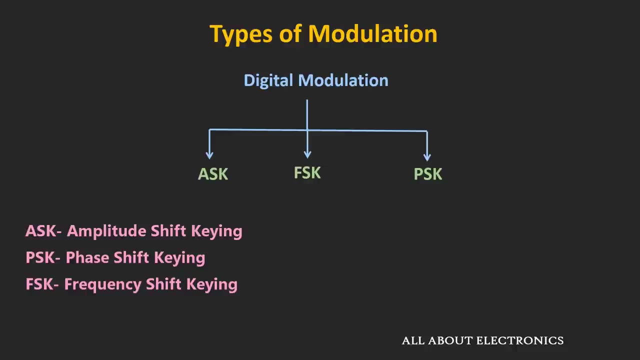 Where the message signal was in analog in nature. Similarly, let's briefly talk about the sum of the digital modulation techniques. So in a very broad sense, mainly there are three different techniques, That is, the amplitude shift keying, the phase shift keying and the frequency shift keying. 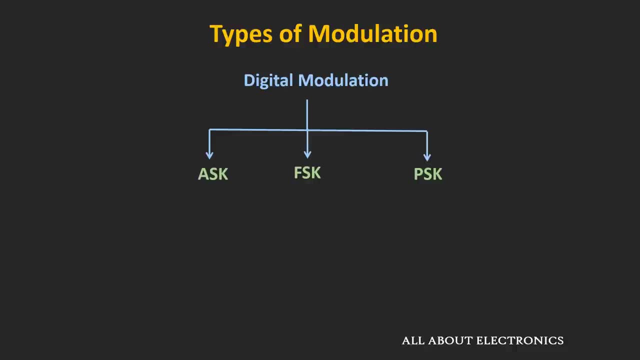 So in all these digital modulation schemes The message signal is in digital form. So this amplitude shift keying is one form of digital amplitude modulation where the amplitude of the modulated signal changes according to the digital bitstream. So in this scheme the binary signal 1 is represented by the fixed amplitude of the